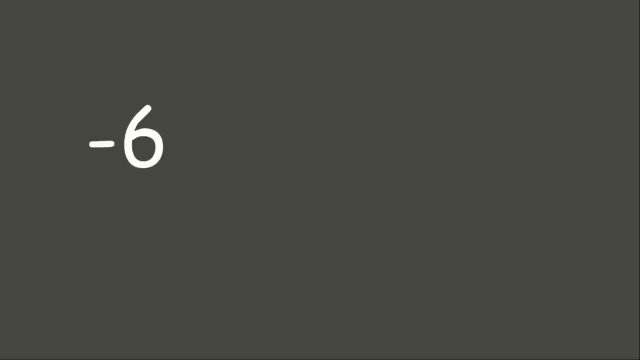 Great job. Now let us try to solve this. We have negative 6 plus negative 4.. Again, let us remember: when we are adding negative integers, we simply add the numbers and copy the negative sign. Therefore, 6 plus 4 is 10.. And copy the negative sign. we will get negative 10.. 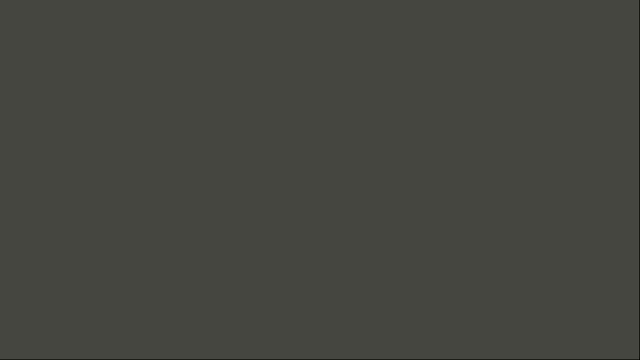 Now let us try to answer this without using numbers and counters. We have negative 10 plus positive 5.. When we are adding opposite signs, first is we need to disregard theuesto sign First is we need to disregard the signs We are going to make 8 or 12, 8i numbers or these points to be positive? 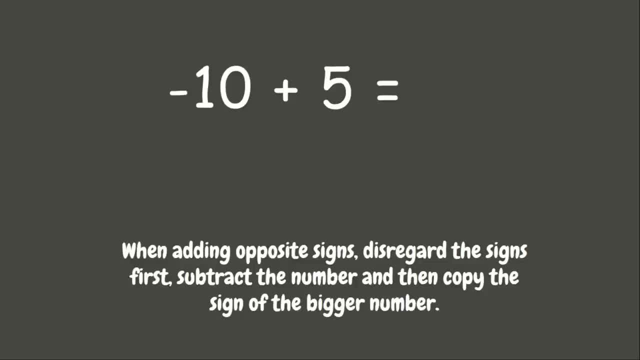 We will also use in the responder which we will add without�를ing, these 4 as negative sign and diversity 0 as negative sign. Where is the reward to end by? We are going to solve these problems, the signs we are going to ignore, whether they are positive or negative, and then 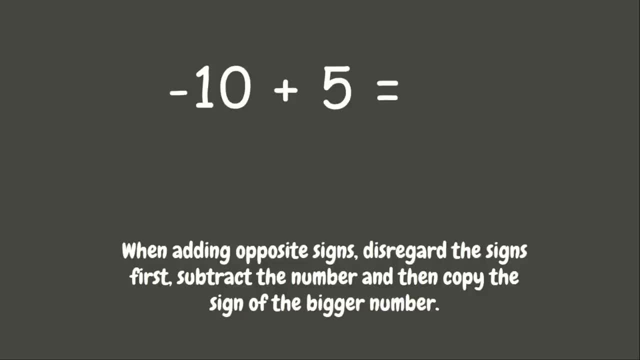 we need to subtract the numbers. here we have 10 and 5, so let us subtract it: 10 minus 5 is 5, and then after that let us copy the sign of the bigger number. when we are looking for the bigger number, we will also disregard or ignore the signs. 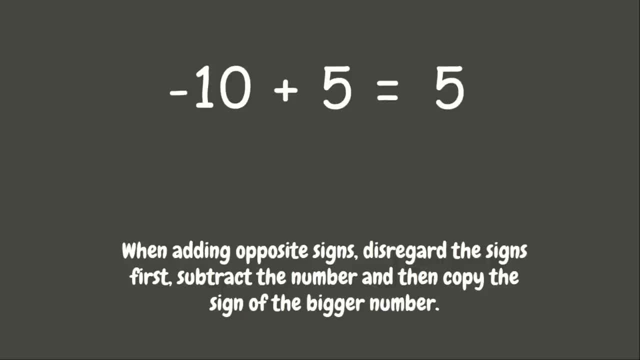 so we have your 10 and 5 and we know that the bigger number is 10. since 10 has negative sign, our answer will also be negative. it means that negative 10 plus positive 5 equals negative 5. now let us check our answer using our 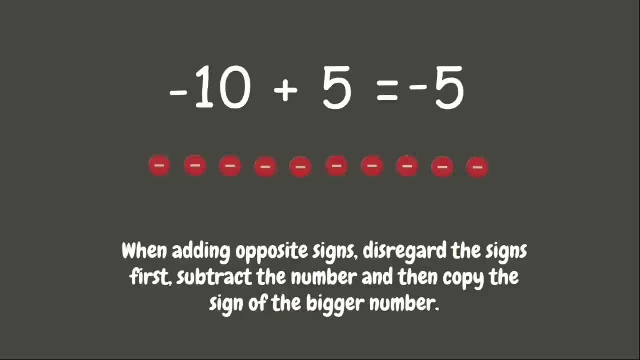 counters, we have 10 negatives plus 5 positives. again, we need to remember that a pair of one negative and one positive is equal zero. now let us cancel the pairs there. now we have 5 negatives left. therefore, our answer is correct. now let's have another example. let us try to solve negative 7 plus. 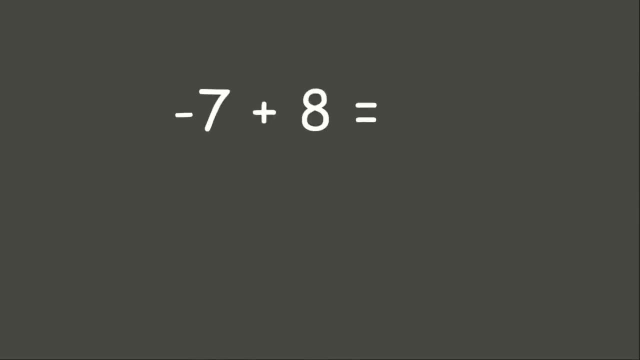 positive: 5, 8. again, we are going to disregard whether they are positive or negative. let us subtract the numbers: 8 minus 7 is 1. now let's take a look at the sign of the bigger number. here, the bigger number is 8 and since it is a positive integer, 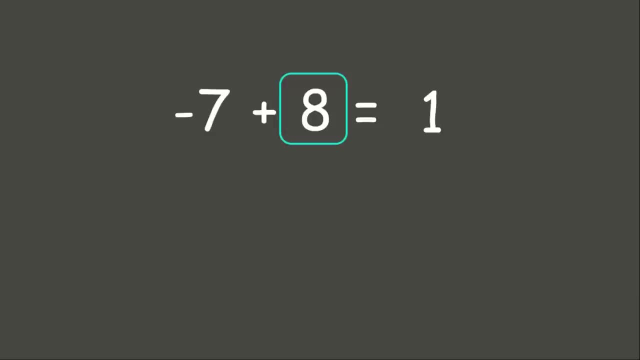 our sum or answer, should also be positive. therefore, negative 7 plus positive 8 equals positive 1. now let us check. if our answer is correct, we have 7 negatives plus 8 positives. again, we need to cancel out the pair of one negative and one positive. there you go. now we have one positive left. therefore our 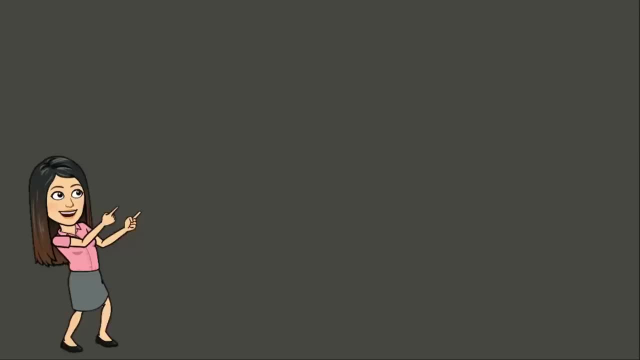 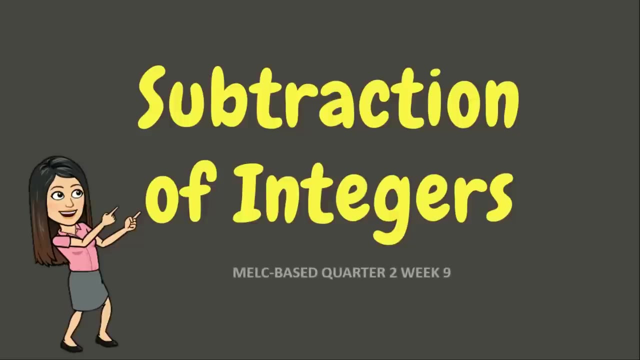 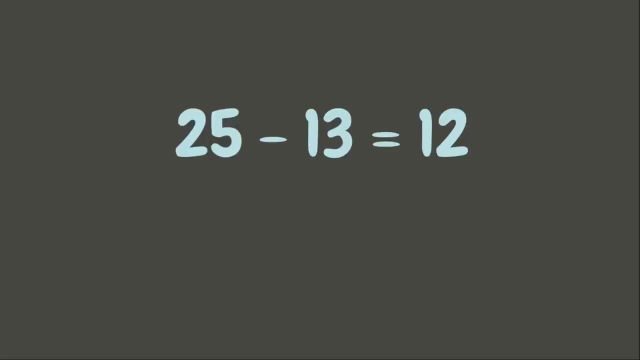 answer is correct: 2, 1 negative, 7 plus positive 2, which means negative, 3. pozyена is positive: 0, 2 and we can definitely say we are both positive and negative if we have negative 1, 0, 3 negative, 6, positive, 7 plus negative, 3.. 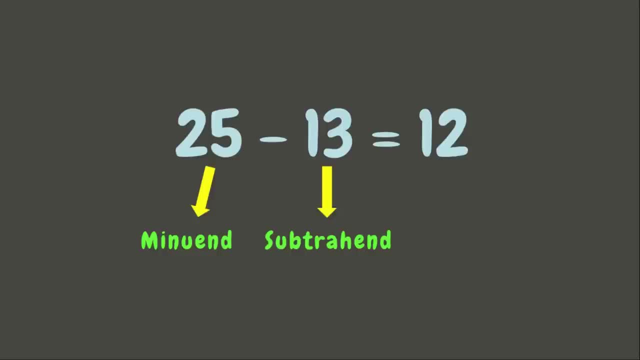 negative 1, 1 negative, 4 positive, 5 positive, 2 positive, 2 minus and minus 2 are wedged off in fin total, while the answers are called different. now that you have recalled the parts of subtraction, you are now ready for our lesson. let's go, let's try. 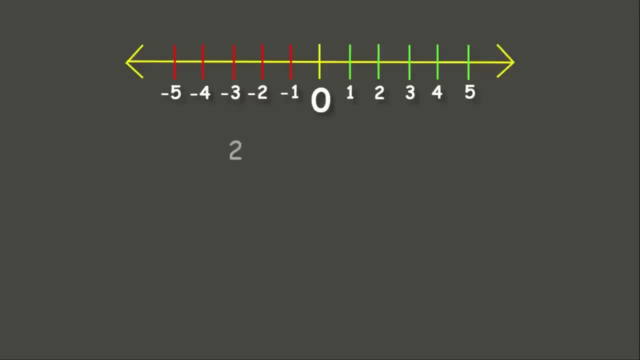 to solve our first example. we have here positive 2 minus positive 1. I know that you already know the answer to this, but let me show you how to solve this using our number line. here, the menu in, or the first number is positive 2 and we need 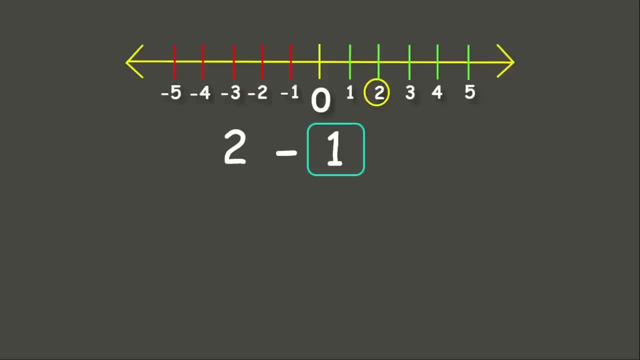 to subtract positive 1 from it. in addition, we learn that if the number is positive, we need to vote units to the right, and if it's negative, we need to book to the left. but since subtraction is the opposite of addition, here, instead of moving this positive into the right, we are going to move to the left. and if 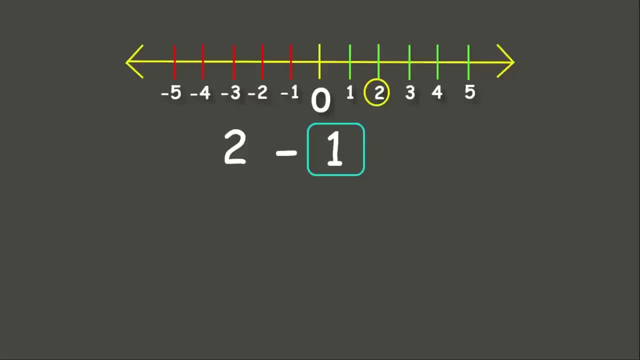 it's negative, we will move to the right. let's have an example: here we have the super hand. positive 1. it means that we need to move one unit to the left. there you go now. our answer is positive 1. this means that 2 minus 1 equals 1. 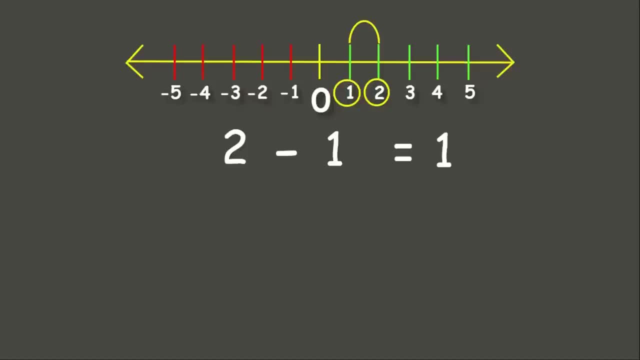 very good. now let us try to answer this using our counters. here we have J, two positive and we need to cancel out or subtract one positive. therefore, we have one positive left- awesome. this means that when we are subtracting positive integers where the minuend is greater, 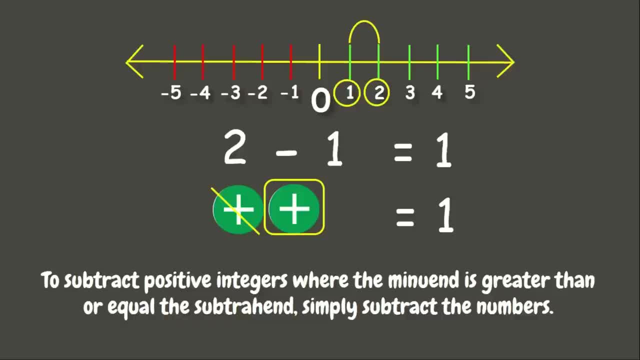 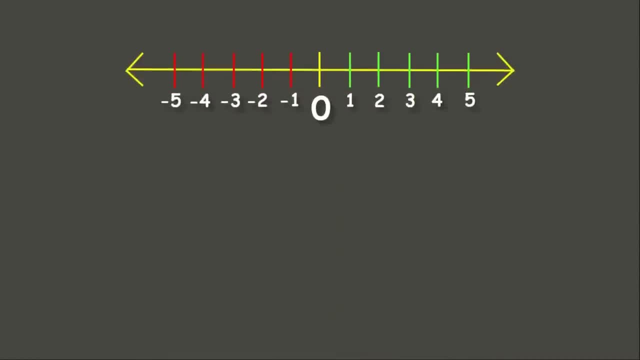 than or equal to subtrahent. we will just simply subtract the numbers. let's have another example. this time we have positive 2 minus positive 3. as you can see, the minuend here is smaller than the subtrahent. but let us try to answer this using our number line. we have the minuend. 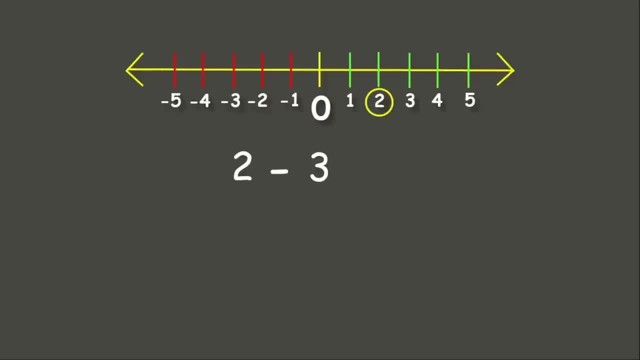 positive 2 minus the subtrahent positive 3. again, since this is positive and we are subtracting, we will move three units to the left. therefore, our answer is negative one. this means that two minus three equals negative one. now let's try to solve this using our counters. we have two positive and we need to cancel out three positive. 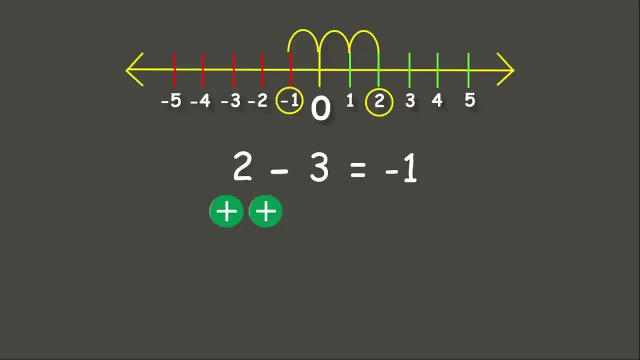 from it. we have two positive and we need to cancel out three positive from it, but, as you can see, we only have here two positive. this means that we need to borrow. we need to borrow from zero. as you remember, a pair of 1 positive and 1 negative is equal zero. 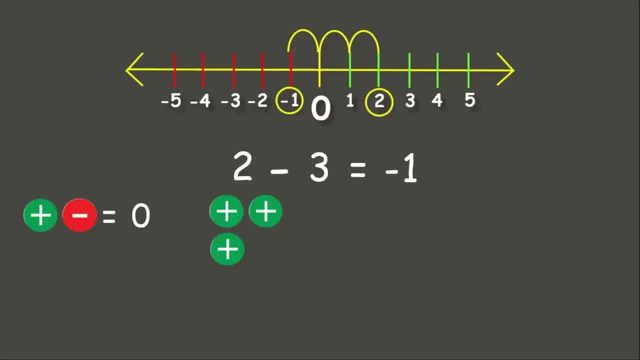 now we can add a pair of 1 positive and 1 negative here, so that we will have 3 positive at this point. we can now cancel out three positives, and now we have one negative left. therefore, our answer is the same, which is negative one. wonderful. now how are we going to subtract? 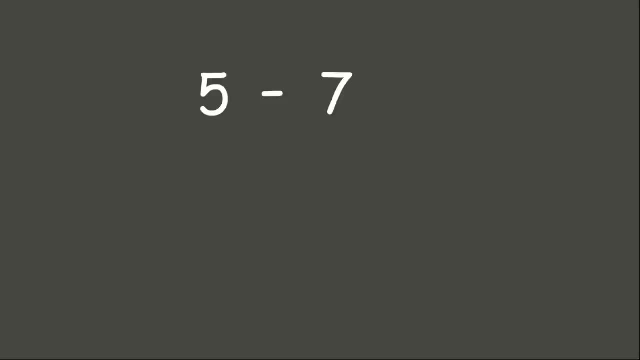 without using any number line or counters. we need to remember that when we are subtracting integers, the first thing that you need to do is to change the operation into addition. so let us change minus sign to plus sign. there you go, and then the next step would be to get. 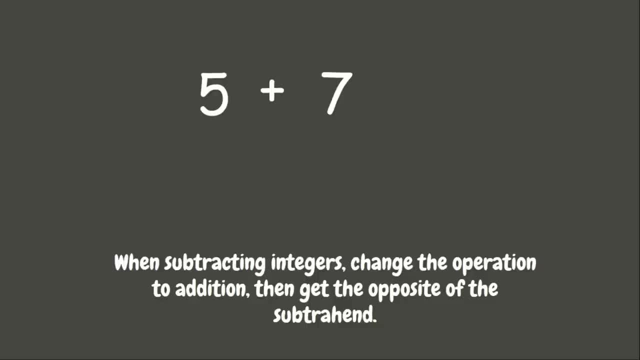 the opposite of the subtrahend. here we have positive 7 and the opposite of positive 7 is: yes, you are correct, it is negative 7. at this point we are now having the operation of addition. this time we need to follow how we add integers when we are adding. 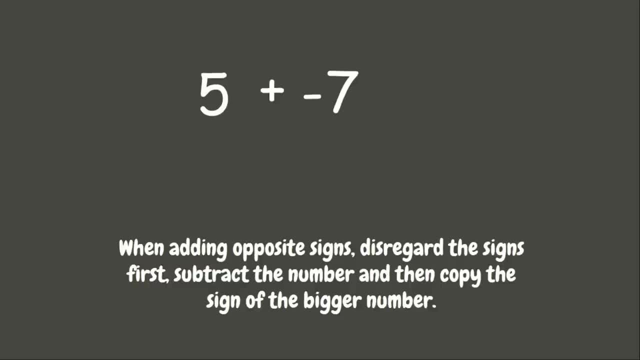 opposite signs. first is to ignore or disregard the sign and then subtract the number. so we have here 5 and 7. now let's subtract 5 and 7, we will get 2, and then, right after that, we are going to copy the sign of the bigger number. 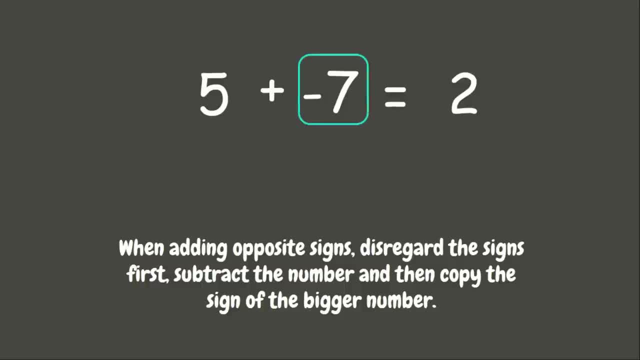 here the bigger number is 7 and its sign is negative. therefore, our answer is negative 2.. now let us check our answer using our counters. so we have five positives plus 7 negatives. now let's cancel out the pairs there. now we have two negatives left. therefore, our answer is correct. 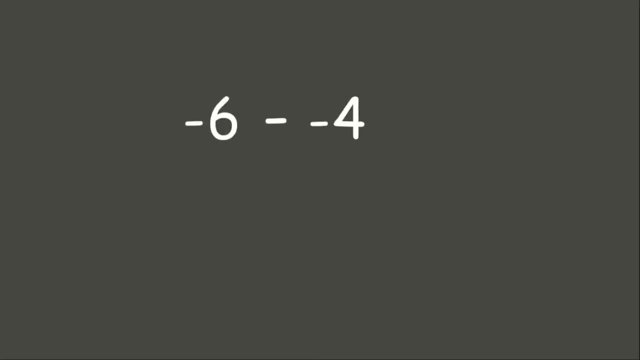 now let us try another one. this time we are subtracting both negative integers, so we have negative 6 minus negative 4.. we're going to subtract negative 3 now. this time moves, we subtract both negative integers. we have negative 6 minus negative 4. 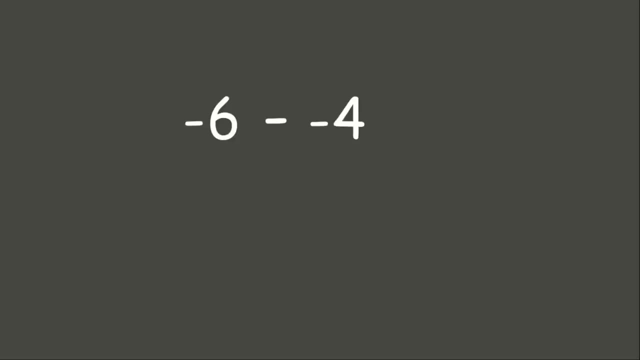 again, again. we need to remember that when we are subtracting integers, the first step is to change the operation into addition. now let us change the minus sign into plus sign. there you go. and then the next step is to get the opposite of the subtrahend. here our subtrahend is negative 4, and we all know. 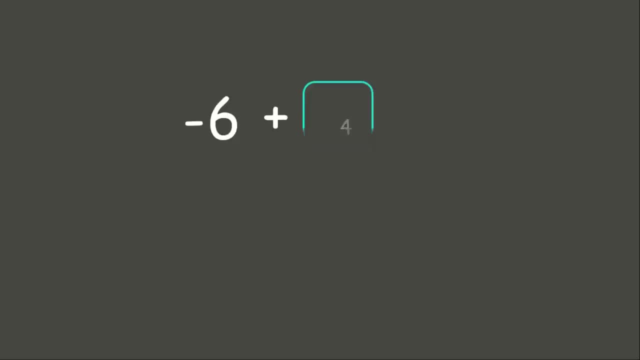 that its opposite is positive 4. now let us add this one. as you can see, we are adding opposite signs. therefore, when we are adding opposite signs, we need to disregard the signs and subtract the numbers. so we have 6 and 4. if we subtract them, we will get 2, and then let us copy the sign of the bigger number. 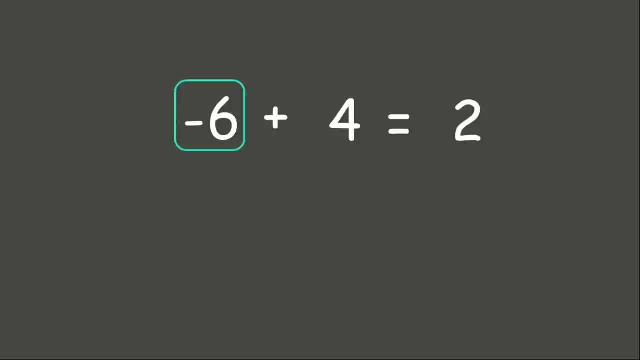 the bigger number is 6 and since it is negative, our answer is negative 2. all right, now let us try to check our answer using our counters. so first we have 6 negatives and then 4 positives. now let's cancel out the pairs there. now we have 2. 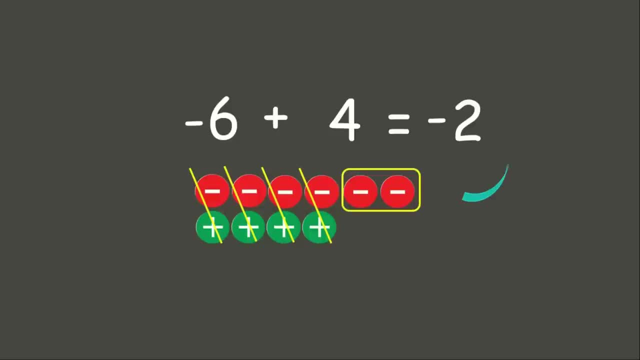 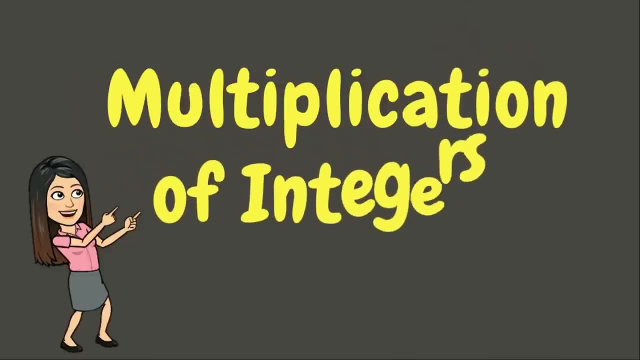 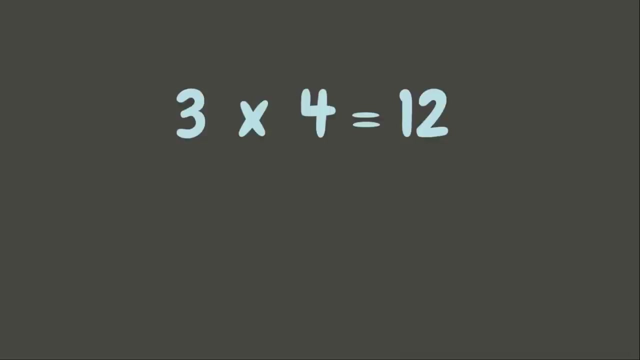 negatives left. therefore, our answer is multiplication of integers. before we begin, let's have a quick recap on the parts of multiplication. the first number for the number that is being multiplied by another number is the multiplication, while the second number, or the number that multiplies the multiplicand, is the multiplier. these two are called factors. 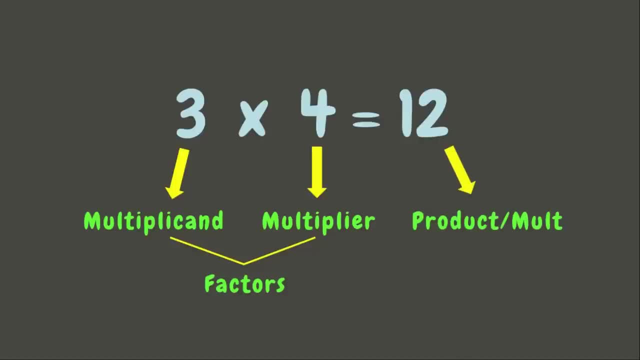 while the answer is what we call the product or the multiple. wonderful, now that you already have reviewed the parts of multiplication, you are now ready to start our lesson. so first one: we have here negative 5 times negative 2 again. we need to remember that when 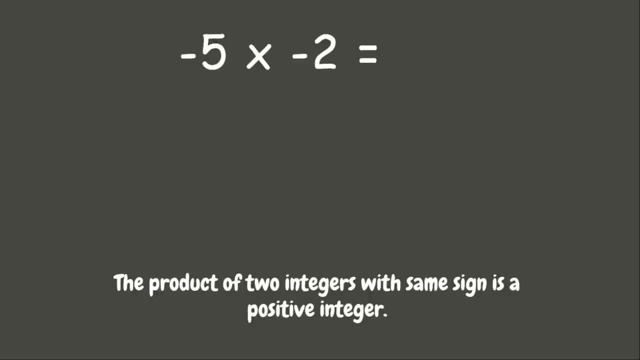 we are multiplying two integers with the same sign, the answer is a positive integer. so since these are both negative integers, we simply multiply them 5 times 2 is 10 and they are both negatives, so the answer is positive. next one: we have negative 8 times negative 4. so let us multiply them 8 times 4 is 32. and since they 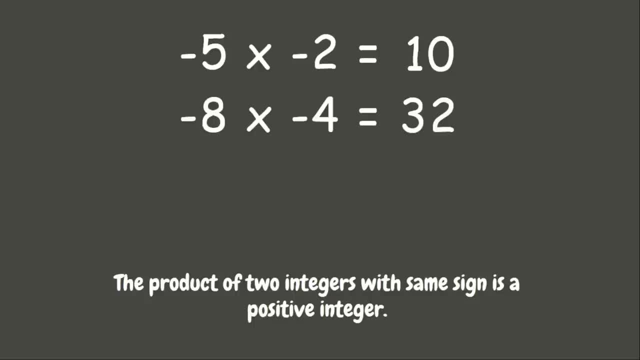 have the same sign, the answer is positive. next one: we have positive 6 times positive 5, so the answer is 30. and since they have the same sign, the answer should be positive. next one: we have here positive 1 times positive 9. if we multiply them, we get positive 9. awesome job. 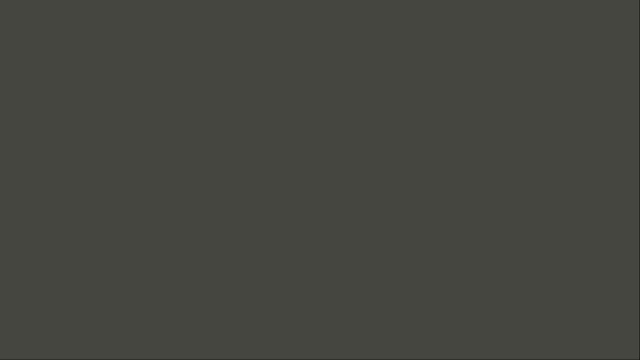 now let's try a different example. this time we will try to multiply two integers with different sign. we have our first one, which is positive 5 times negative, 2 again. we need to remember that when we are multiplying two integers with different signs, the answer must be a negative integer. 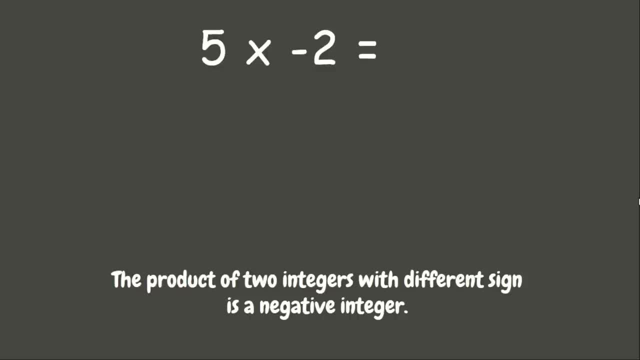 so let's multiply 5 times 2 is 10, and since they have different sign, the answer is negative 10. next one: we have negative 7 times positive: 4. 7 times 4 is very good, it's 28. and since the factors 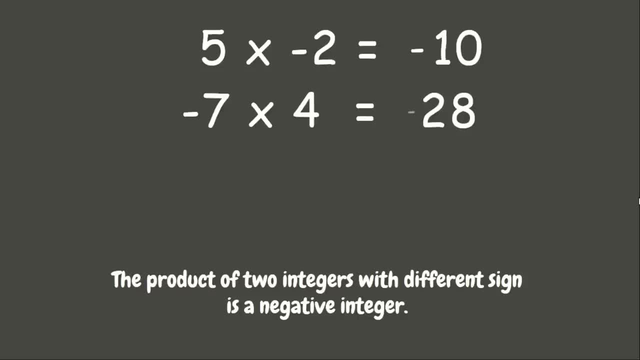 have different sign, the answer is negative. next one: we have negative 6 times positive, 10 6 times 10 is 60, and since they have different sign, the answer is negative. for our final example, we have here positive 5 times negative, 9, which is 45, and. 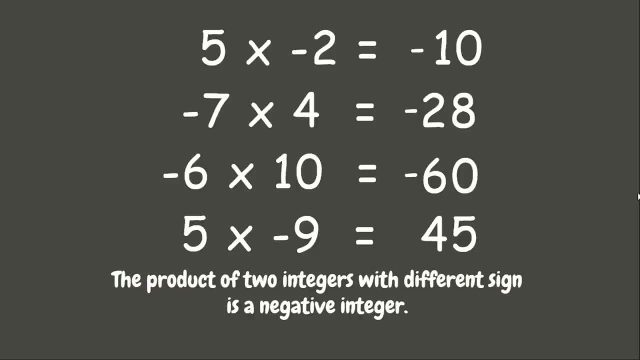 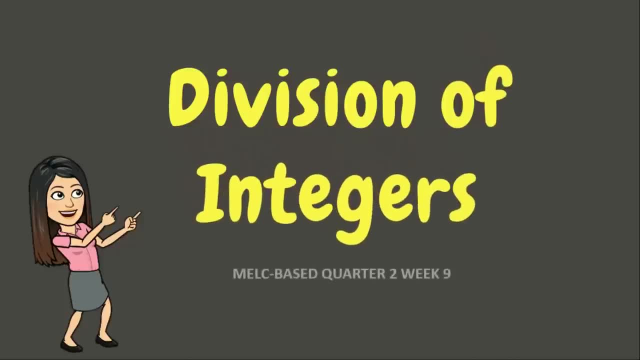 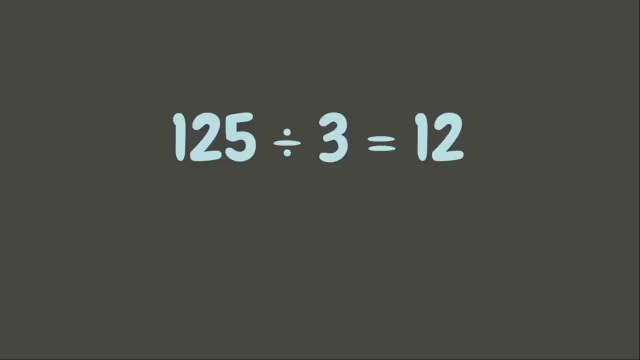 again, since they have different signs, the answer must be negative. First, let's have a quick recap on the parts of division. The first number, or the number that is being divided, is called dividend, while the second number, or the number that divides the dividend, is the divisor, and our answer is what we call. 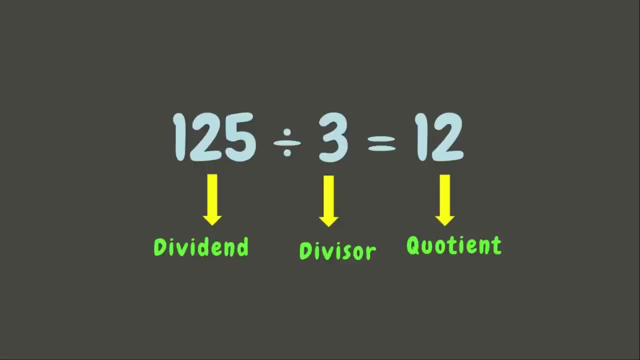 the quotient. Now that you already know the parts of division, you are ready for our lesson. So our first example is negative 18 divided by negative 3.. Again, let us remember that when we are dividing integers by the same sign, the answer is a. 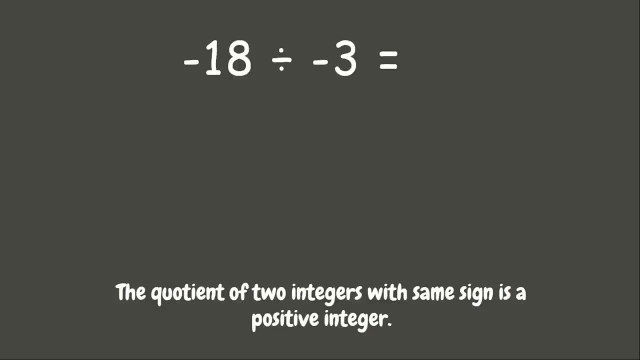 positive integer. Here we are dividing both negatives, Therefore our answer will be positive. So negative 18 divided by negative 3 is Very good. it's positive 6.. Now let's try another one. We have here negative 20 divided by negative 4.. 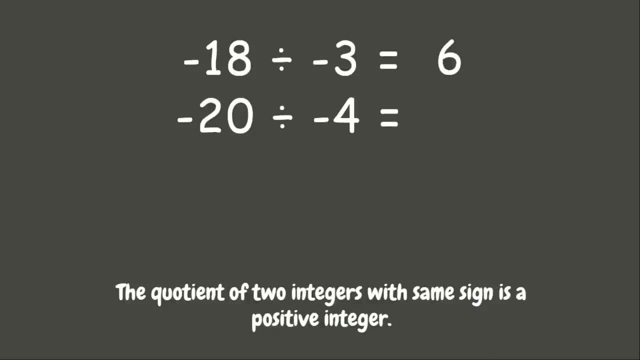 Since they are both negatives and they have the same sign, our answer must be positive. Therefore, negative 20 divided by negative 4 is Correct. it's positive 5.. Next one: we have positive 8 divided by positive 2.. 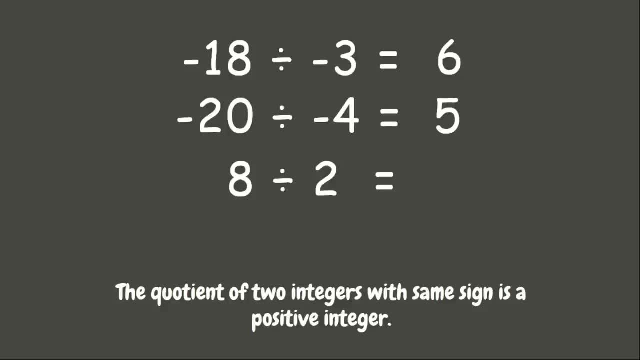 Since they are both positive integers, this means our answer must be positive. So 8 divided by 2 is Positive 4.. And last one, we have Positive 14.. Positive 14 divided by positive 7. What is your answer? 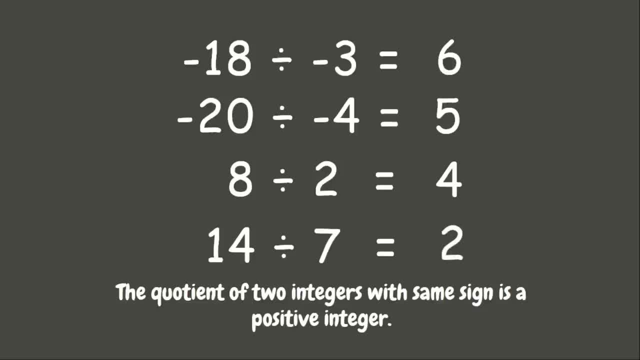 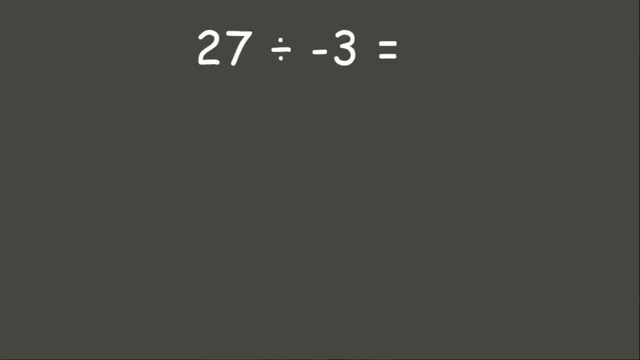 Great job. it's positive 2. Awesome. Now let's try a different one. This time we are going to divide different signs. Our first example is positive 27 divided by negative 3. Again, you have to remember That when we are dividing two integers with different sign, the answer is a negative integer. 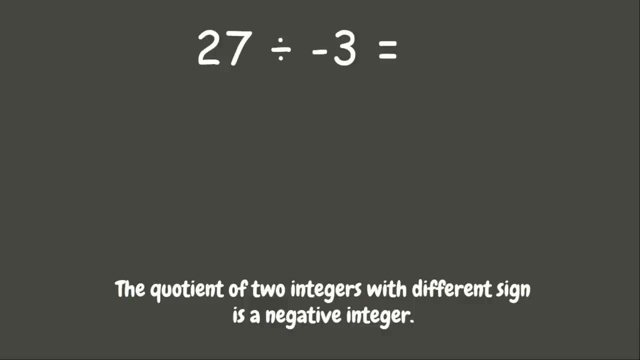 Therefore, 27 divided by negative 3 is 9.. And since they have different sign, let us put the negative sign. Our answer is negative 9.. Next example: we have here negative 12 divided by 4.. So let us divide first the numbers. 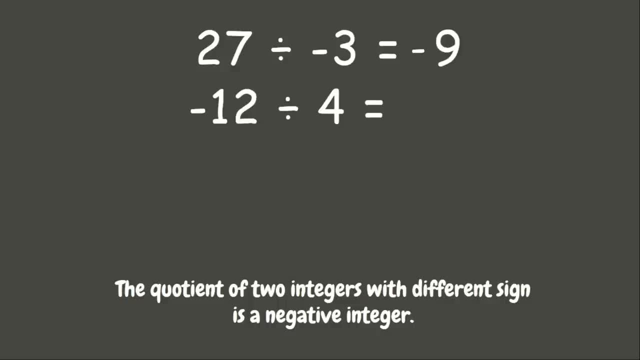 12 divided by 4 is Very good: it's 3.. And since they have different sign, the answer must be negative. Next one: we have negative 28 divided by positive 7.. Good job, it's 4.. 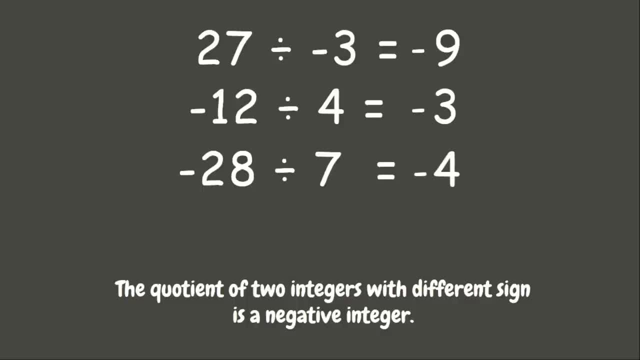 And since they have different sign, the answer is Negative. Let's try another one. Lastly, we have here negative 34 divided by the positive 17. What is your answer? Wow, you are correct, It is negative 2..